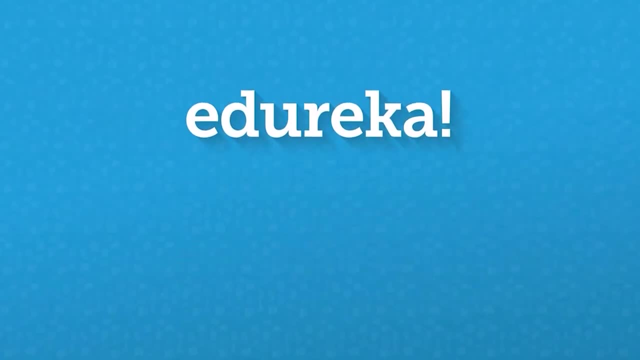 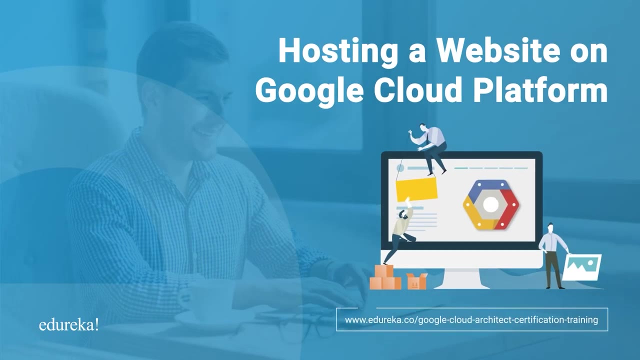 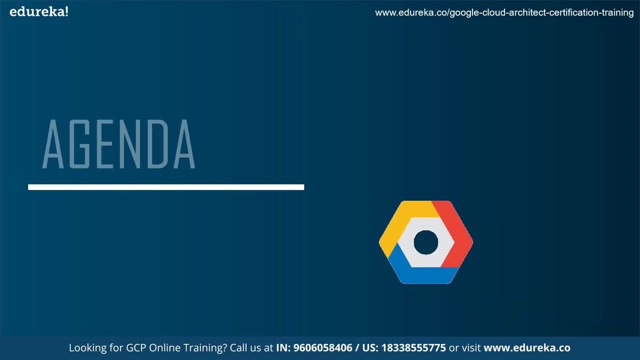 Hi guys, this is Kaurav from Betureka. Welcome to today's session on hosting website on Google Cloud Platform. Now, before we get started on the topic at hand, let's just discuss today's agenda first. The first thing we talk about is: what is website hosting, followed by why? 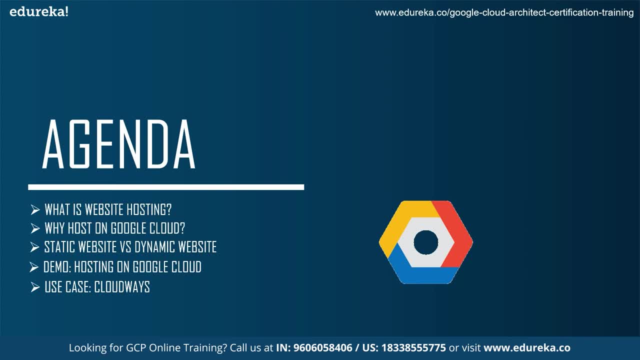 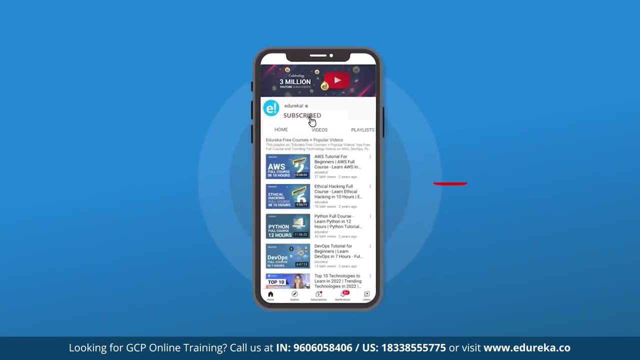 we host on Google Cloud, Then we come to static website versus dynamic website, Then we have a demo on hosting on Google Cloud And finally we have a use case on Google Cloud hosting, which is on Cloudways. So let's get started. And also, if you do like our videos, please do. 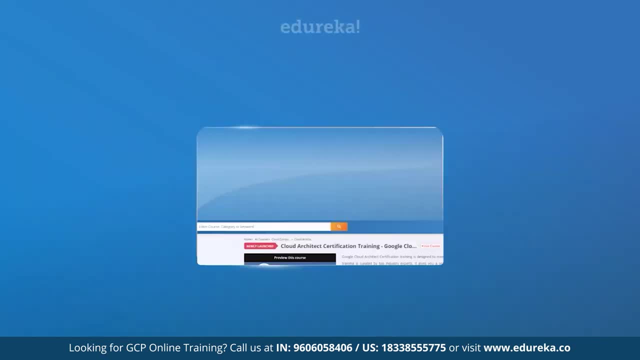 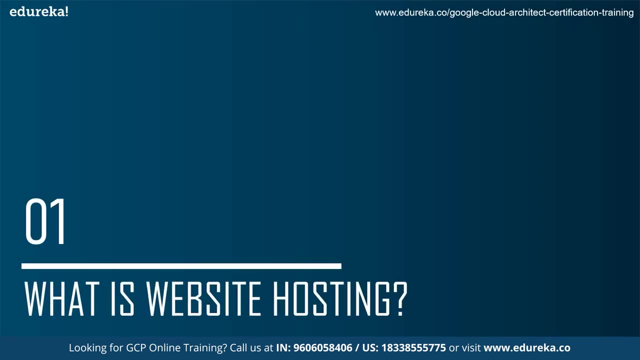 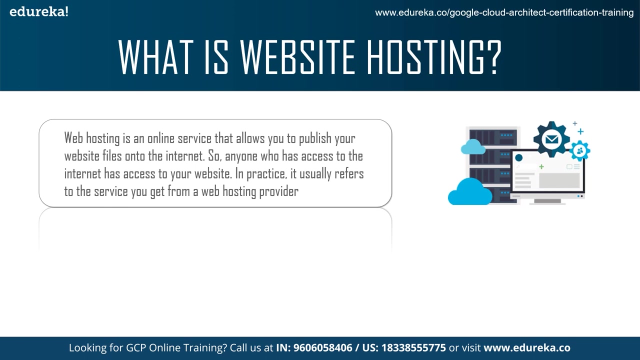 subscribe to the Betureka channel And if you're looking for a GCP certification, please do check the link in the comments below. So the first topic is: what is website hosting? Now, when we talk about website hosting, we can see that website hosting is basically an online service. that 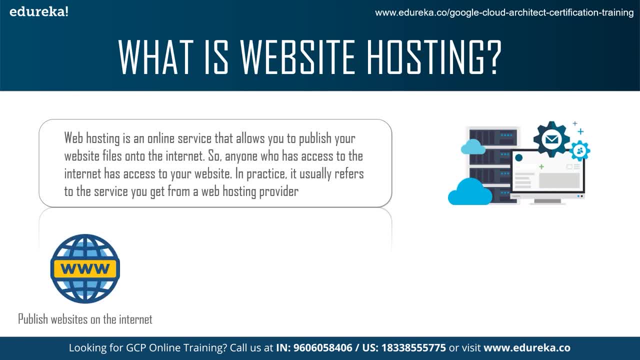 allows you to publish your website on the internet. So anybody who has access to the internet has access to your website And basically in practice it refers to service you get from a web hosting provider. So a hosting provider is somebody who is a third party and basically 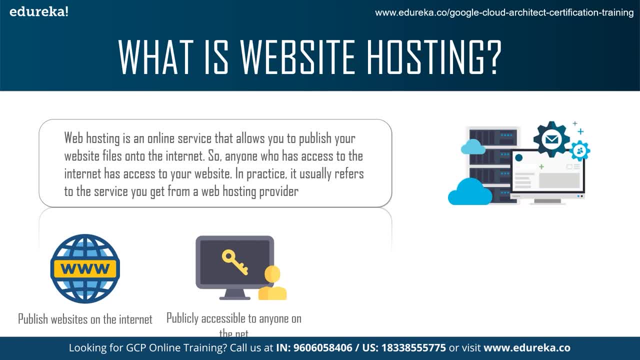 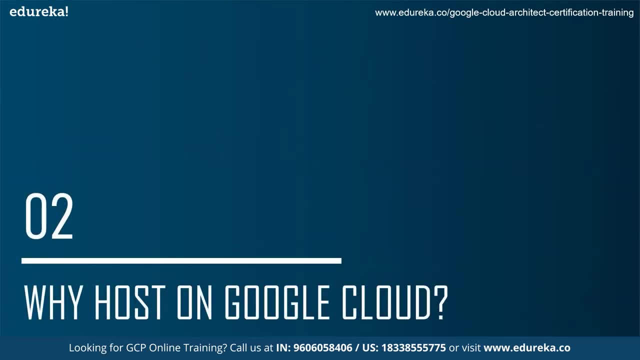 helps you host your websites for you and maintains them right. So hosts are responsible for maintaining the site. Next up, we talk about why host on Google Cloud Right? So there are various reasons why you should host on Google Cloud. There are various. 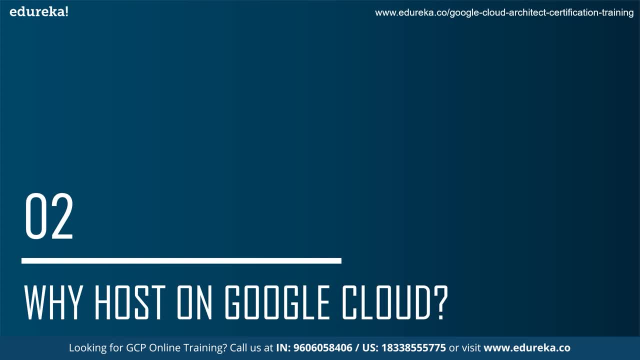 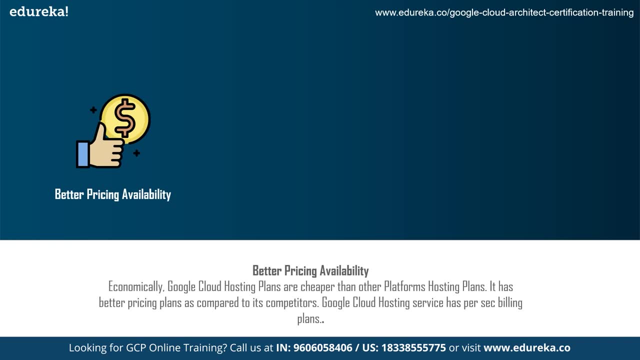 advantages. as to why people use Google Cloud platform for hosting, The first reason is the fact that it has a better pricing availability right. So when it comes to better pricing availability, economically Google Cloud hosting plans are much cheaper than the AWS or Azure. 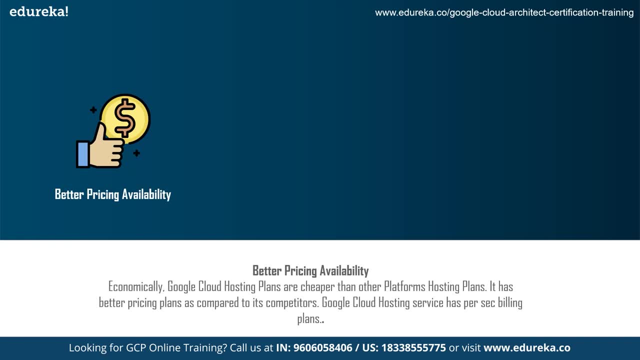 hosting plans Like Google Cloud platform is definitely at least 5% cheaper than Azure and at least 8% cheaper than Azure. So when it comes to better pricing availability, Google Cloud hosting plans are much cheaper than AWS or Azure hosting plans. Right, So this better. 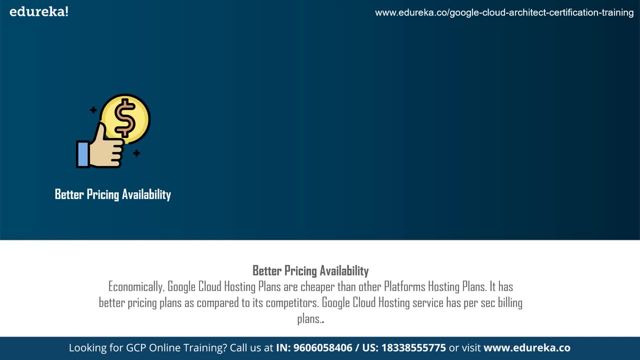 pricing plan is basically something that keeps Google Cloud platform hosting services ahead, and it is built per second, So that is why Google Cloud platform is better pricing. Next up, we talk about the enhanced execution that Google Cloud platform offers us. So when we talk, 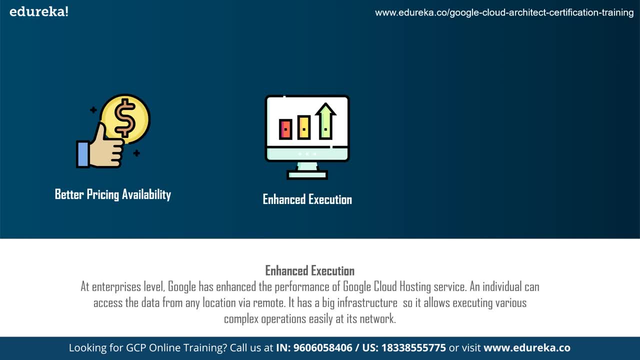 about enhanced execution. we see that the enterprise level Google Cloud has enhanced the performance of the of its hosting services. right So an individual can access the data from any location via remote or a big infrastructure. right So that big infrastructure allows Google Cloud. 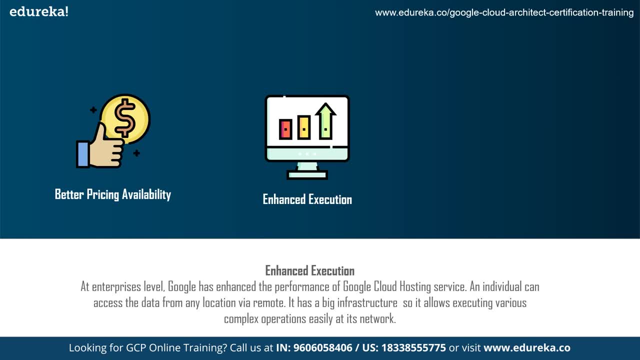 to basically execute various complex operations and enhance its own resources and services. right Next up, we talk about the commitment to constant development. So when we talk about this, we talk about the fact that when Google is developing its infrastructure rapidly, right that is, according to its customer's requirements. 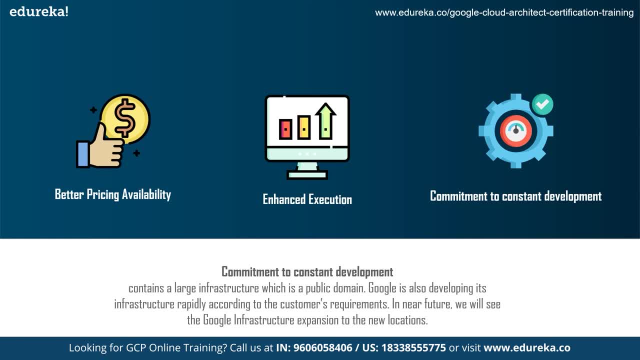 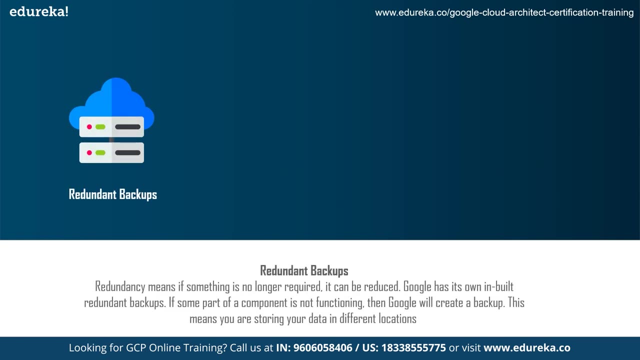 So when, in the near future, we'll see that the customer's requirement has changed, it will be based on the Google infrastructure, based on new locations, right? So it's continuously evolving based on your requirements. Next up, we see that Google Cloud hosting. 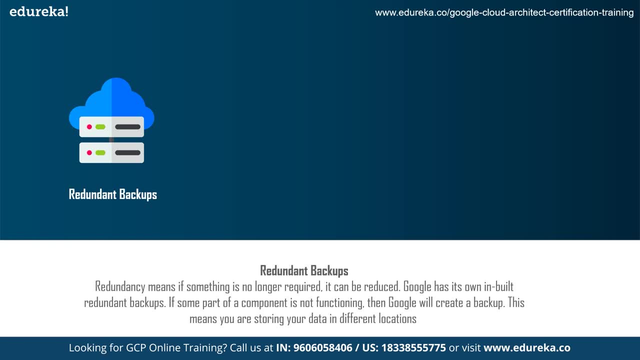 is basically something where you can have redundant backups. Now, redundancy, basically, is something where you do not have an extra copy of certain data, right? So every data is unique to itself, right? So Google has its own built-in redundant backups, right? 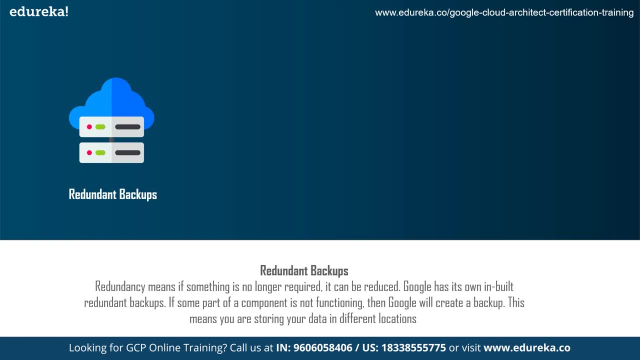 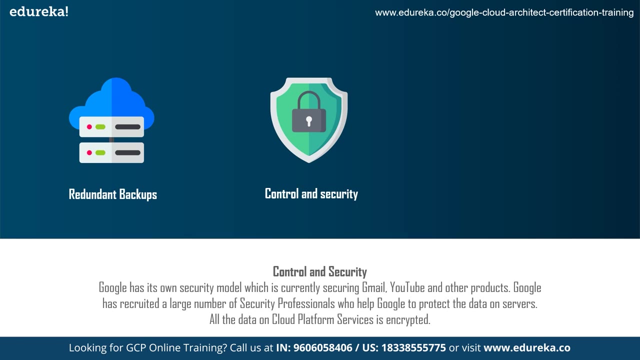 So if some component is not functioning, then Google will create a backup automatically, because you are storing the data in different locations, right? So that is why there's a backup. Next up, we talk about the control and security that Google Cloud Platform hosting will provide us. 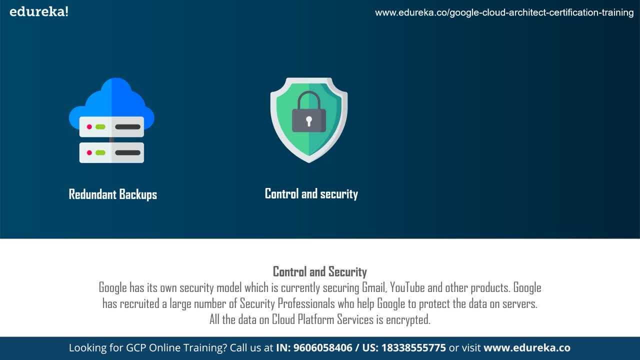 This is because that Google has a backup. Google has its own security model. So when it has its own security model, which is again used in other services provided by Google, such as Gmail, YouTube and other such products, Google has recruited a large number of security professionals. 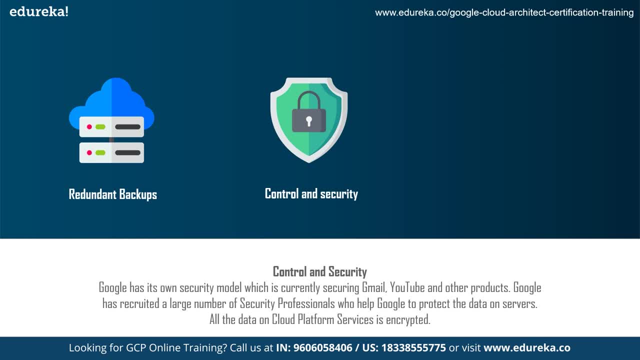 just to basically protect the data of the servers, right? So all the data on the Google Cloud Platform is encrypted, So it is extremely secure. And finally, we come to the fact that live migration of data is possible. So one of the top advantages of Google Cloud hosting. 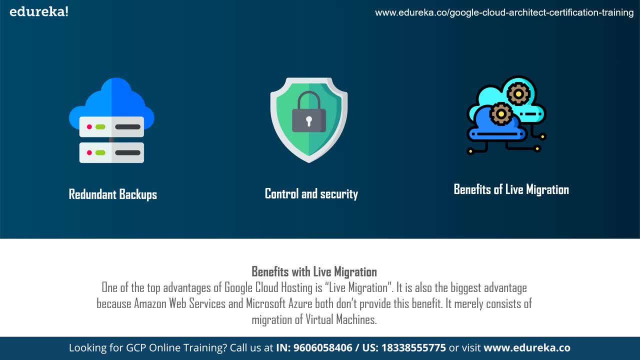 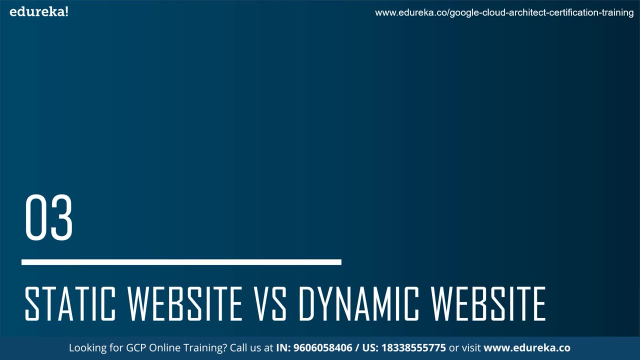 is live migration, right. It is the biggest advantage, because AWS and Azure both do not provide this benefit, right, So it only consists of migration of virtual machines when it comes to AWS. Next up, we talk about static website versus dynamic website. 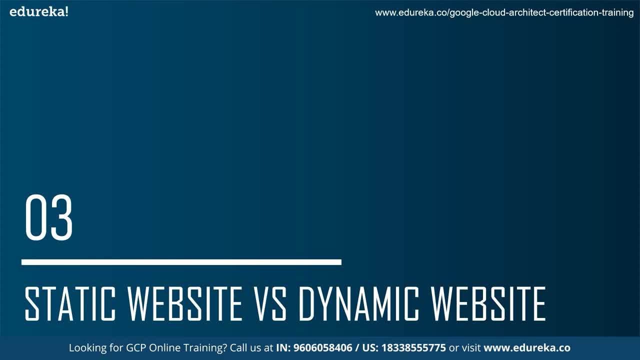 So when we talk about hosting in cloud, that is basically cloud hosting, which is one of the various kinds of hosting available, such as VPS hosting. is it So when we talk about hosting in cloud, that is basically cloud hosting, which is one of the various kinds of hosting available, such as VPS hosting. is it? 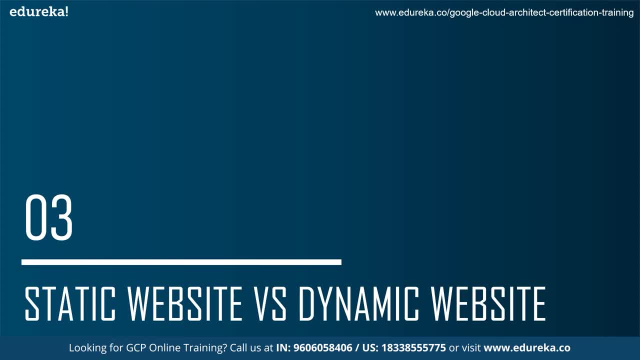 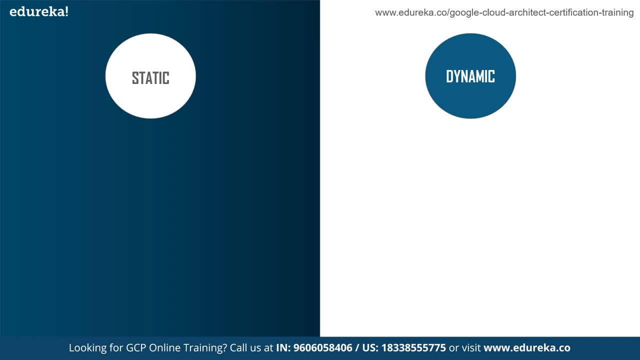 so, when it comes to cloud hosting, there are two kinds of websites that can be hosted right. so one of the websites is a static website and the other is a dynamic website. so when it comes to a static website, it is basically the same info displayed to every user that is there, while a dynamic website will be. 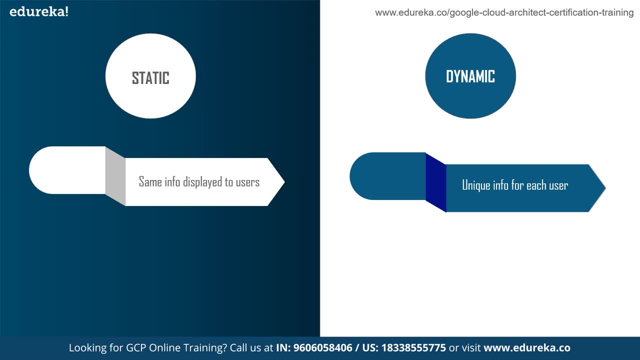 unique for each user. for example, your Gmail login page and your Gmail homepage will be different for every user because it's customized to you and you can customize it as well, whereas a basic HTML hello world page will be the same for everybody, and that is an example of a static web page. next up, we talk about 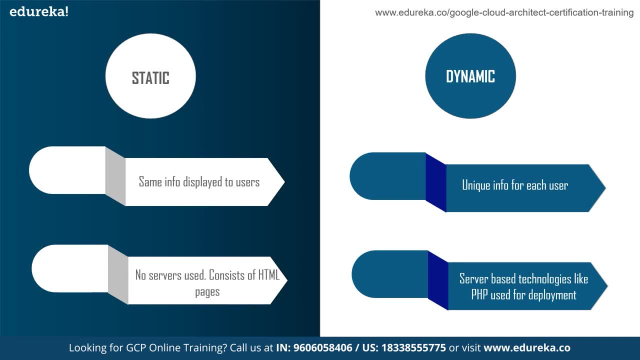 the fact that static web page does not have any servers that are used, right, so it consists of basic HTML pages which can be stored in buckets, and these buckets can then be hosted on Google Cloud using the endpoints, right, whereas dynamic websites need server based technologies like PHP, and that is. 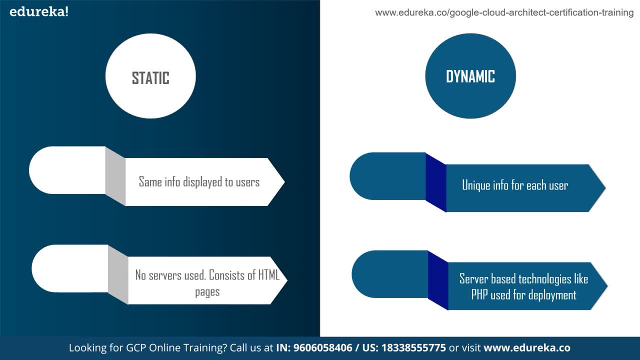 basically what we're going to talk about in this video. so let's get started. basically, something that is necessary for deployment: web apps are used for the deployment of dynamic websites, so these are the two different kinds of websites that are present when it comes to hosting. next up, we have a demo on: 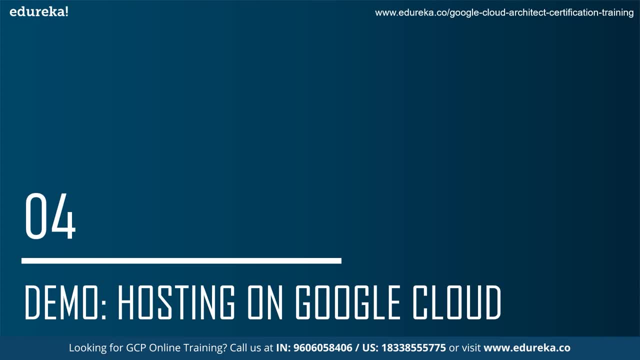 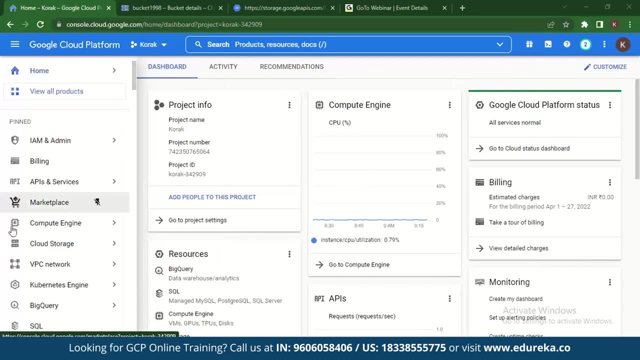 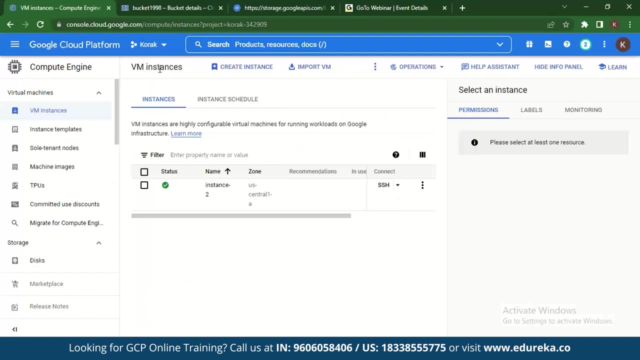 basically how to host a static and a dynamic website on Google platform. so once you've basically logged into your Google Cloud Platform console, you can go to compute engine and go to VM instances. we're going to basically talk about how to host a dynamic website on Google Cloud Platform. 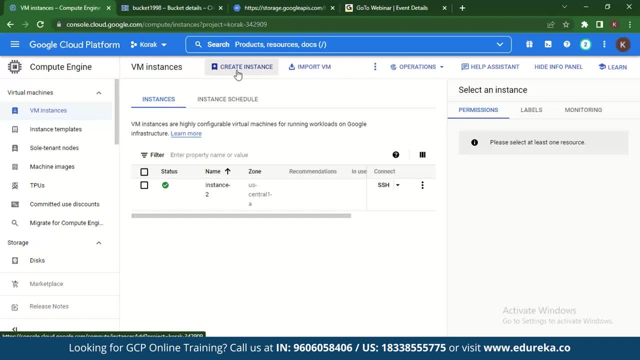 so the first thing you need to do for this is create your own project, and in that project you'll have to go to compute engine and then create an instance. make sure that you have a service account as well, but in this demo will be using the default service account. that's there, so let's get. 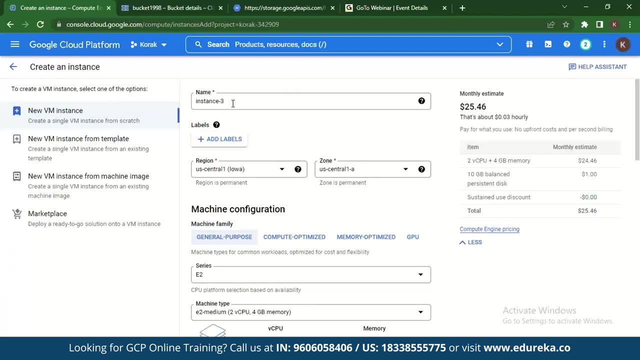 started. so let's see there's an instance name here and it's named as instance 3, so we can go to my instance name here and it's named it instance 3, so we can keep that as is. and on the right hand side you can see that the pricing for 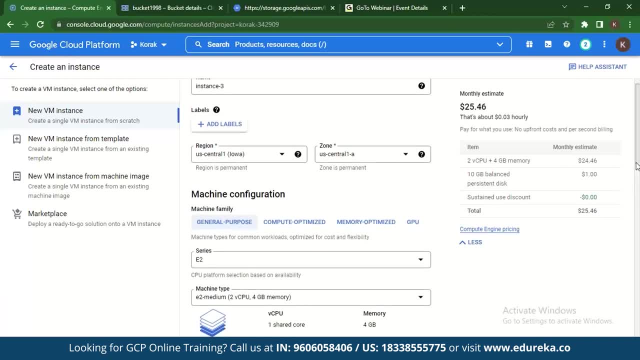 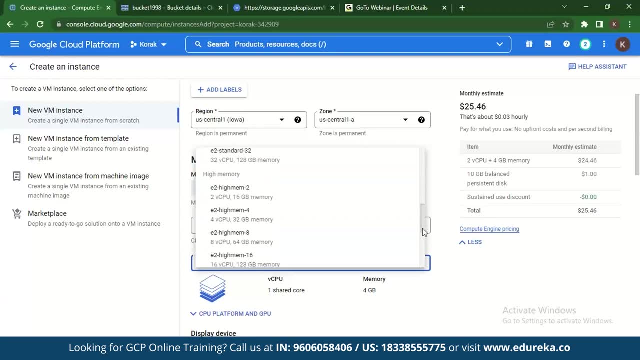 the estimate pricing for our machine is given right. so the pricing depends on the amount of resources you use, the kind of machines you use, and what you have to do here is just get it, change it to n1. so when you change it to n1 you can see. 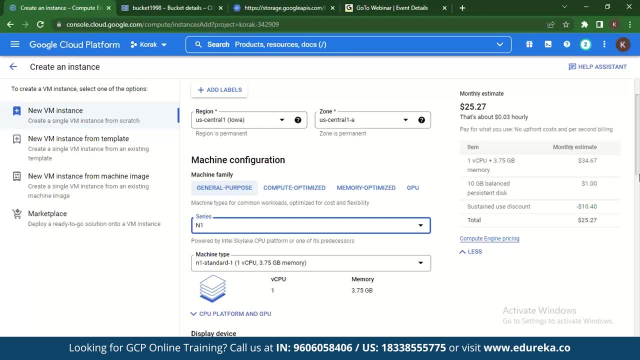 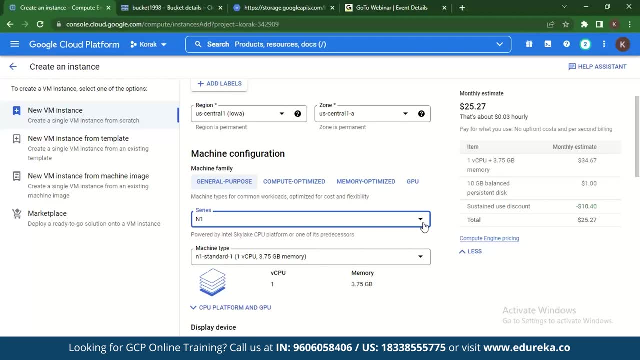 that the price has just reduced or it's the same, because you don't need a lot of users to be logging in to your EM instance right now. it's just you, so you will be the one logging in, so you don't need a very powerful machine. that's n1. 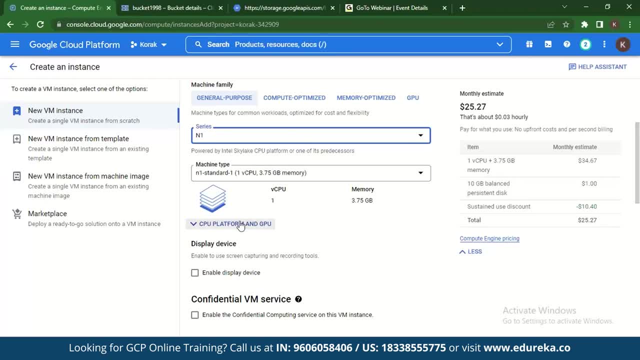 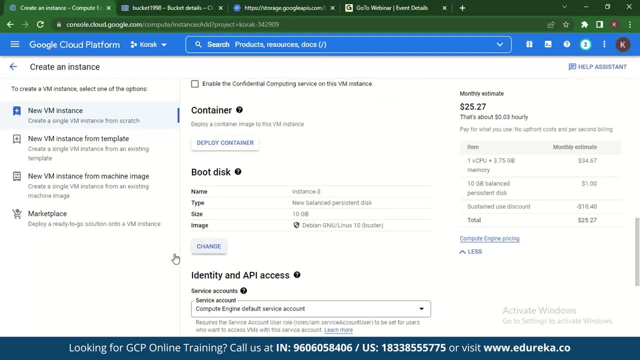 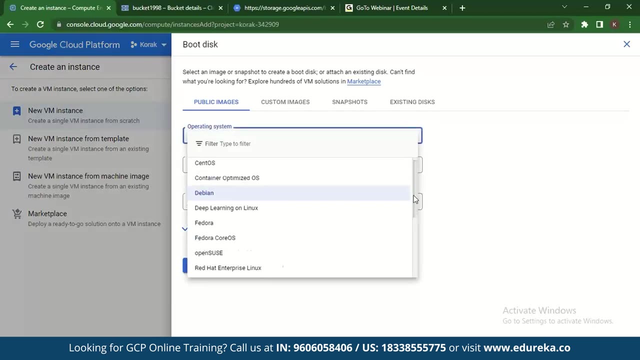 and what you have to do here is to platform, GP, configure all this. it's done and come here and change the boot disk. now can keep it as you wish. you can keep it as devian as well, if you want. i'll be keeping it 2.2. 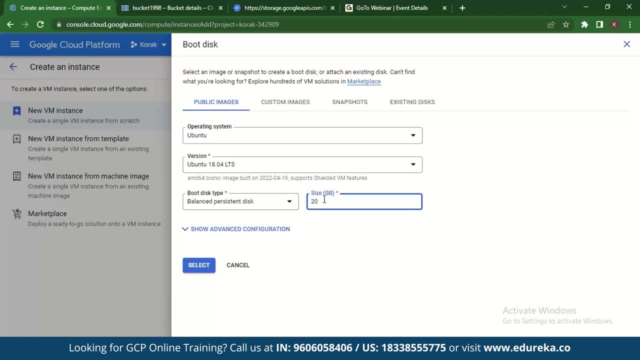 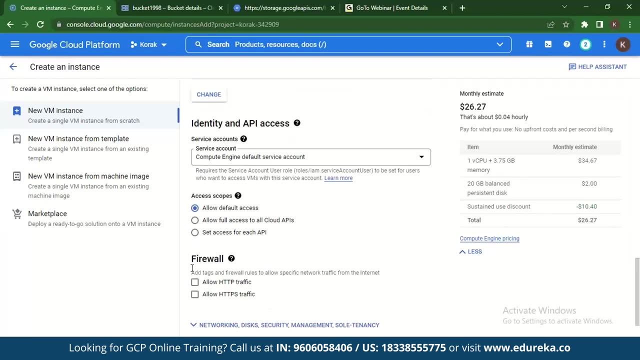 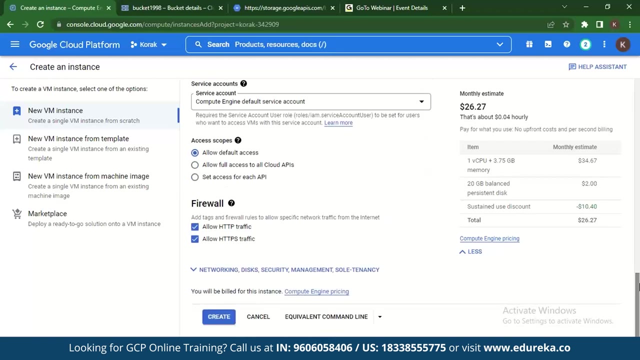 and changing my space to 20 gb- that is, changing my boot disk- and after that you'll have to allow http and https traffic, because you need public access for your website. so when you basically go onto the internet, you want your website to be shown right. so after this, what? 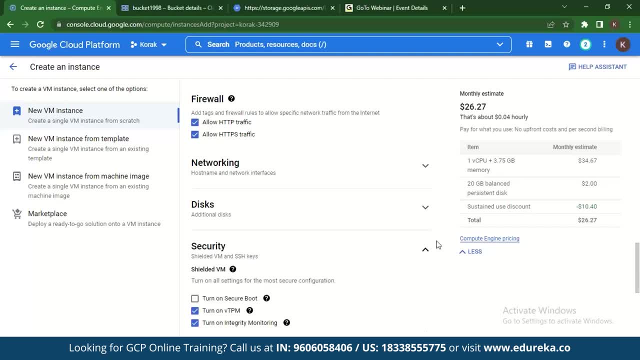 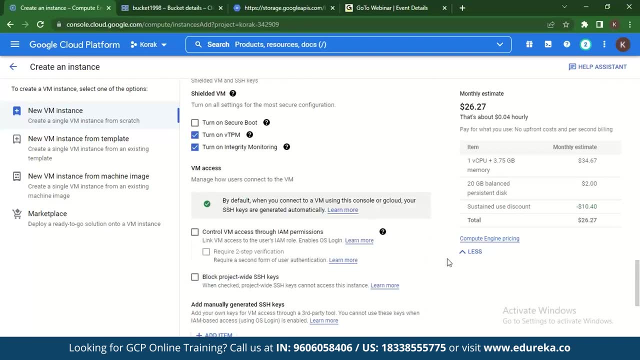 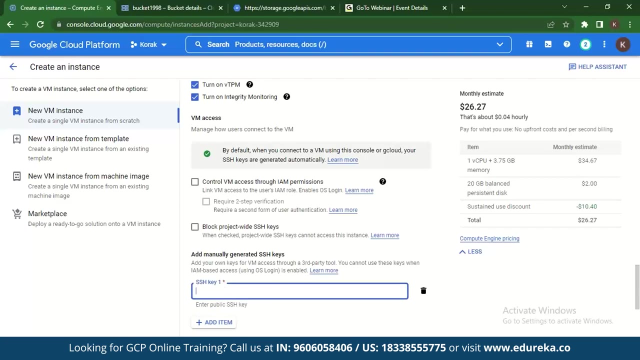 you have to do is basically go to security, and here we have to do is manage your access for the vm right. so for this, what we need to do is create a public key, and you'll have to add the public key separately, and for that we'll be using 40gen. 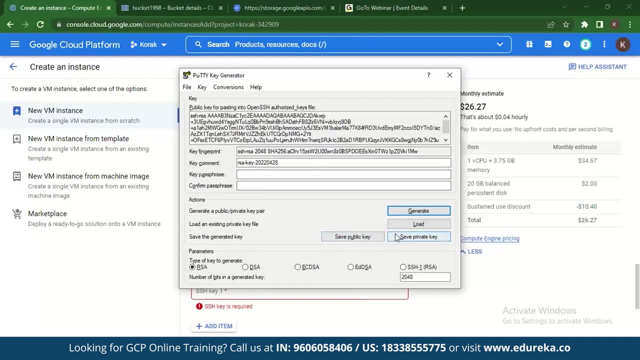 generate your key, save it as private key right, so you'll have to make a passphrase, and that passphrase is for basic authentication and improving the security right, so you can keep this passphrase whatever you want to and save it as a private key. so let's just name this private. 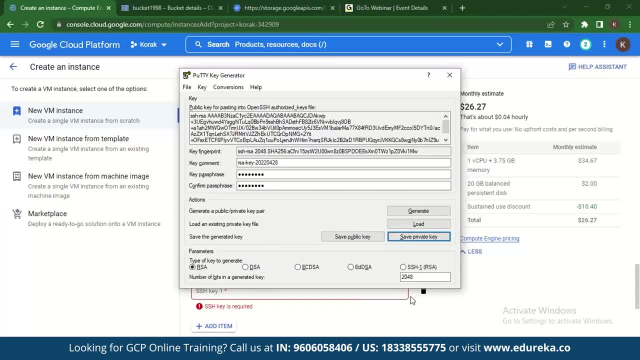 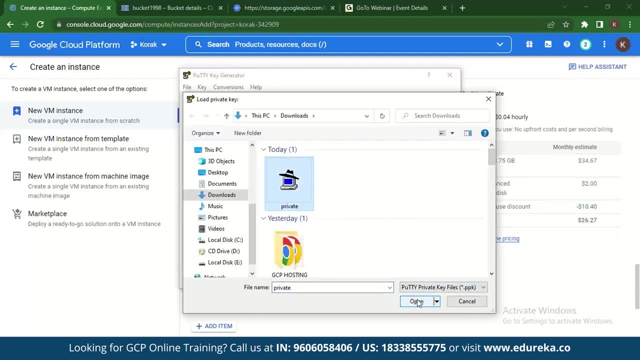 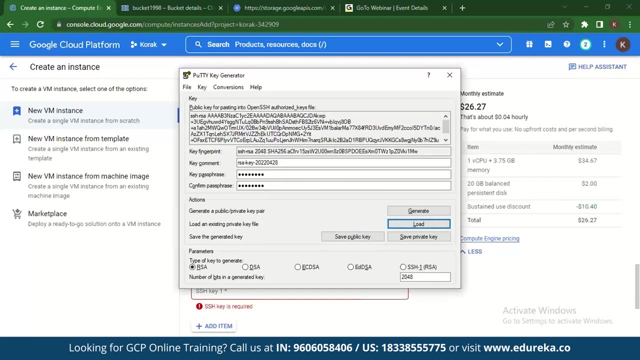 and dot ppk, save that and after this, what you need to do is load this, go to private and open this up. open up your with your passphrase and you'll have your public key that you can copy. you can just copy this and we can now go back here. 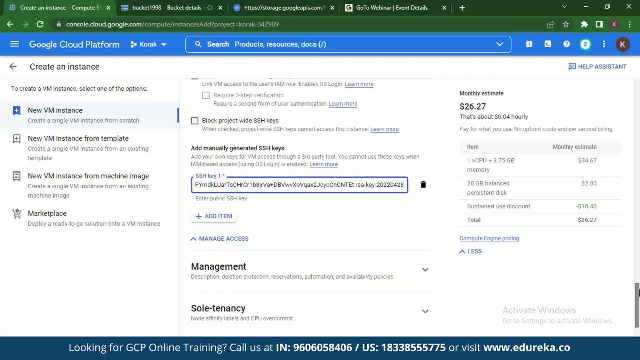 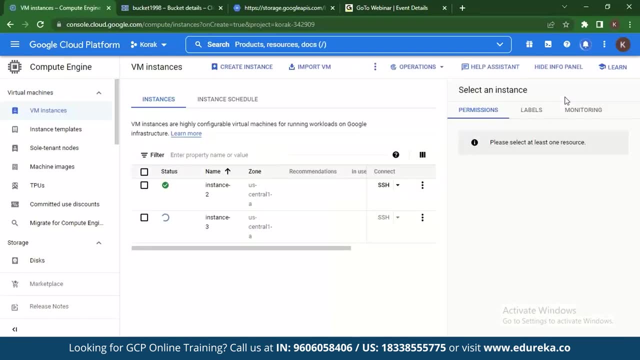 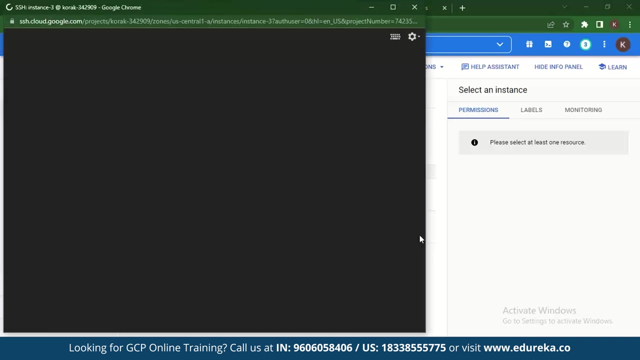 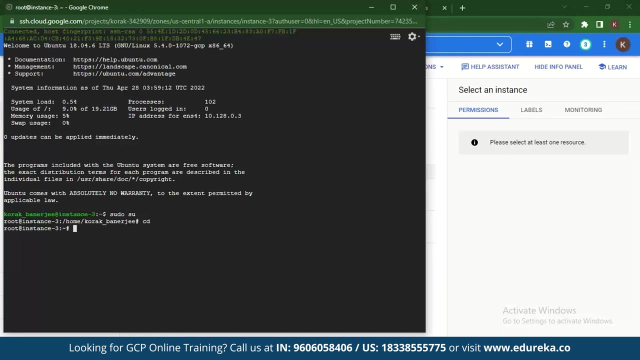 and paste this here and after this, just create the instance. right, so your instance is now created. what you need to do now is connect to the ssh and open it up. now the window, once connection to your ssh has been established, type in sudo, su, and you can just go in there, cd, and just type apt get. 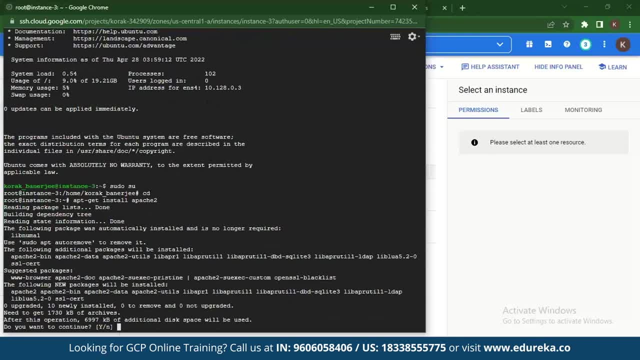 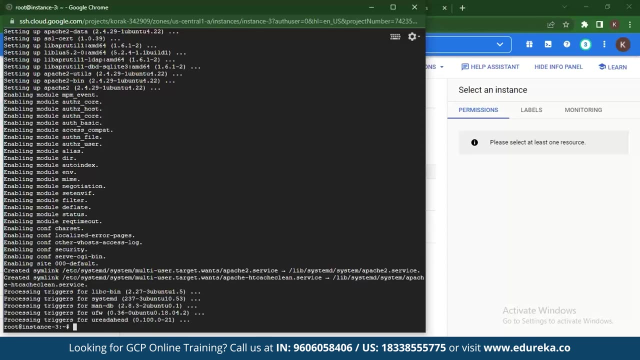 right. so this is what you have to write and you can see your apache 2 is being installed. now apache 2 is basically going to be the server, and just type in y right. so this is now done. so what we can do is just check if our apache is running. for that we just have to do this. 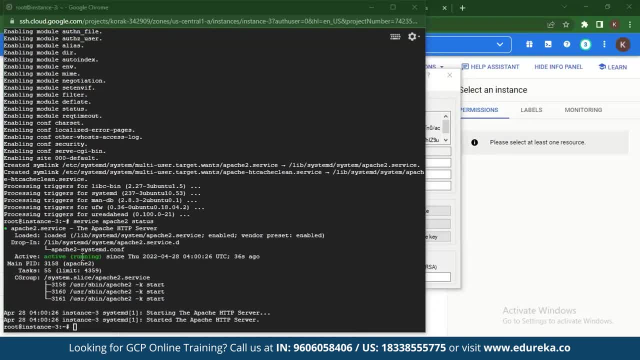 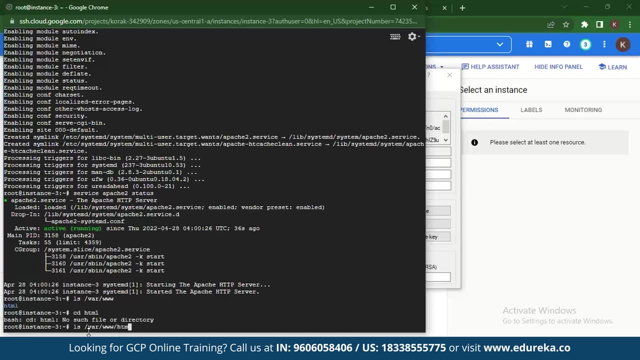 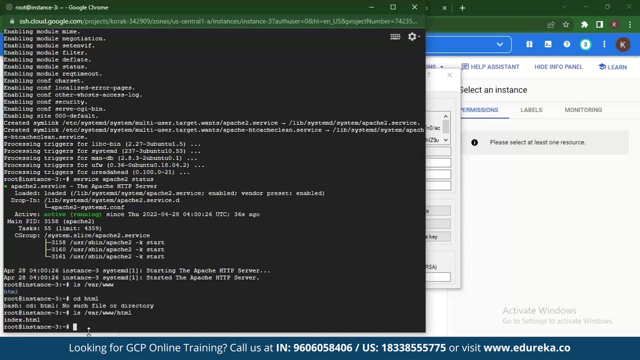 as you can see, basically this is running. so basically what you have to do now is go back in here, type in ls, so you can see that we have the indexhtml page, and then add html here. if you go into the directory you can see there's an indexhtml page. 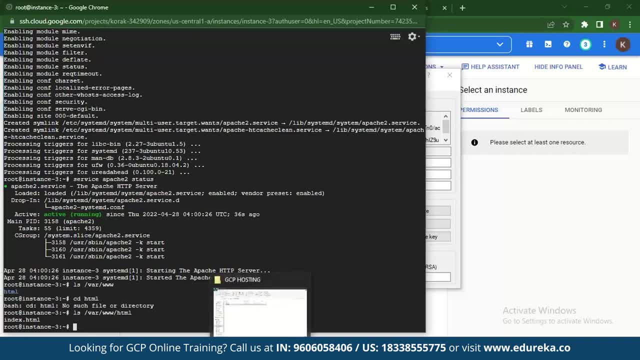 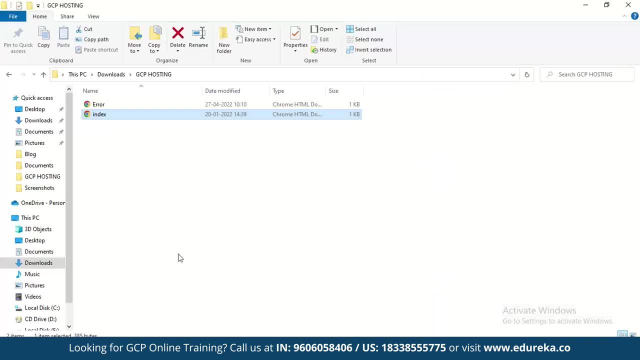 now, when we talk about the indexhtml page, what we have done here is the indexhtml page is supposed to be the apache server page, but we need to host our own website right, our own dynamic website. so what we've done here is had our own indexhtml web page, which is 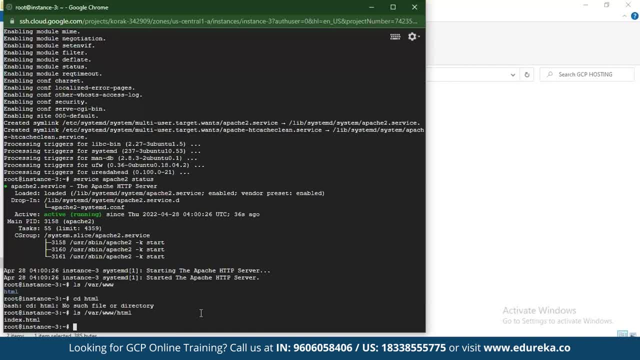 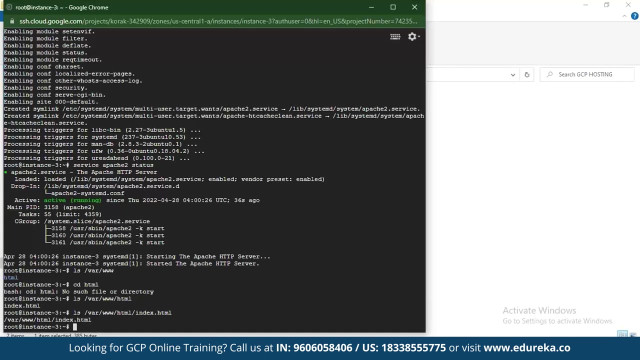 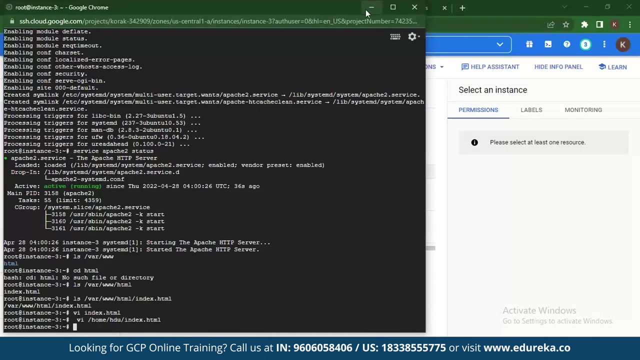 going to replace the apache server web page, right, so let's try that out. go into ls right, do backslash and indexhtml right. so now you're in here and basically what you have to do after this is vi index dot html, the indexhtml page. you take this code in and you change it in the indexhtml. 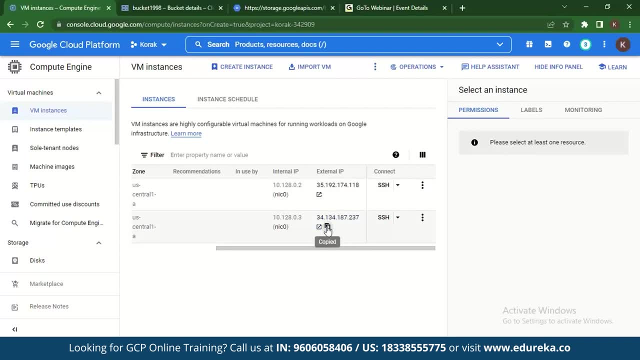 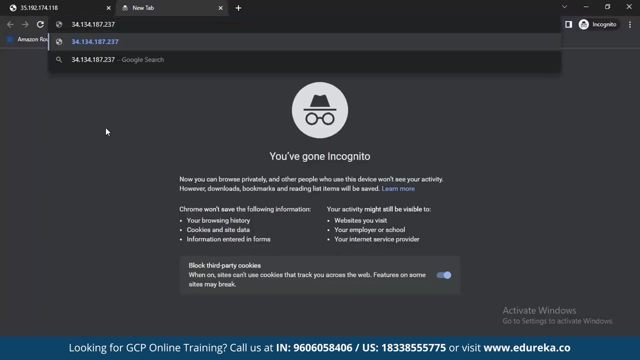 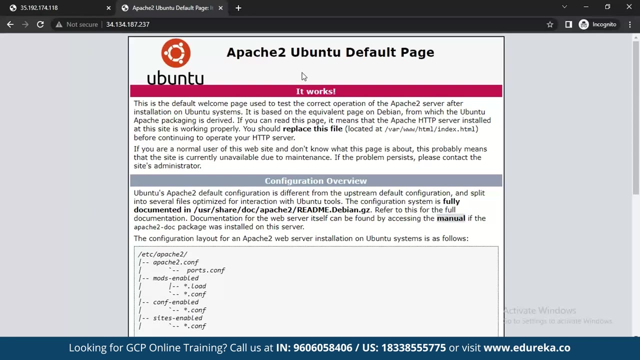 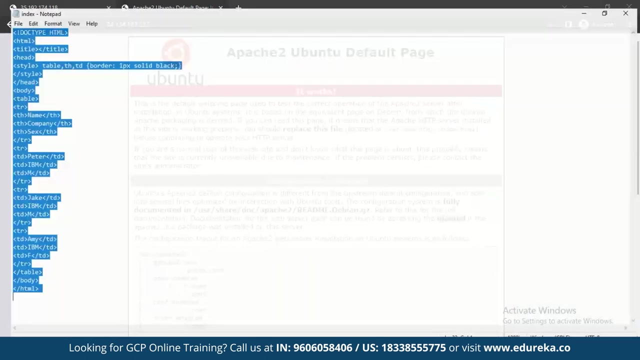 and let's now go back and copy this and once you're done copying, just go back to your incognito so you can see apache server default page. right, so you can see that this page has basically been activated and it's running. what you need to do is change this. this is your code. this is the. 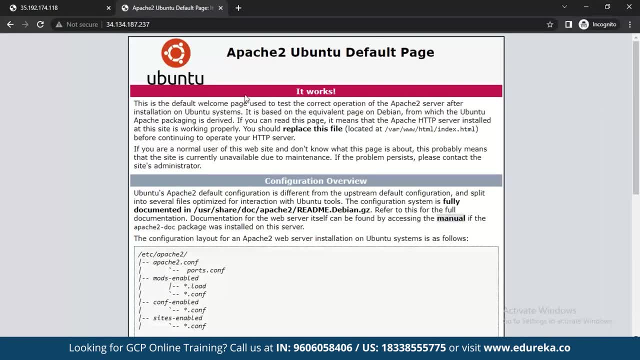 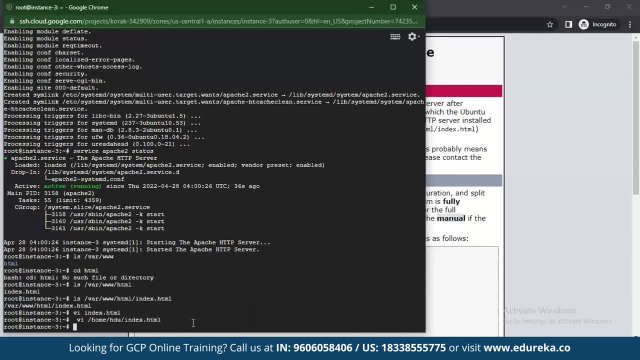 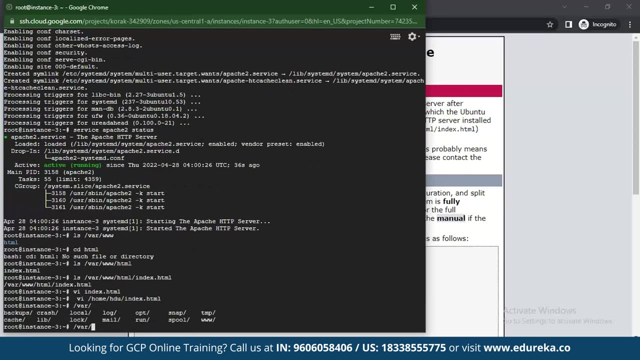 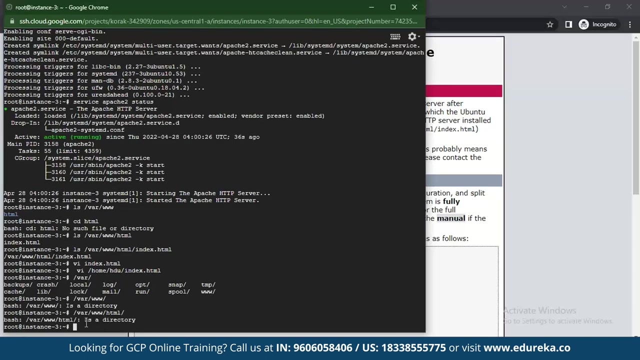 web page with which you will change this page right. so basically, what you have to do is go back into your ssh and into your indexhtml, which is basically just right. so you just go back to right and go to your indexhtml. so basically, you can see that html is already a directory. 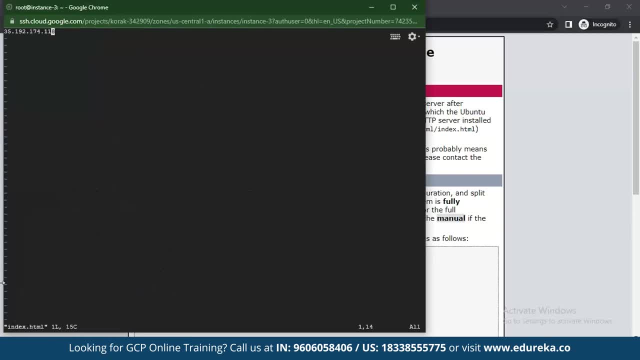 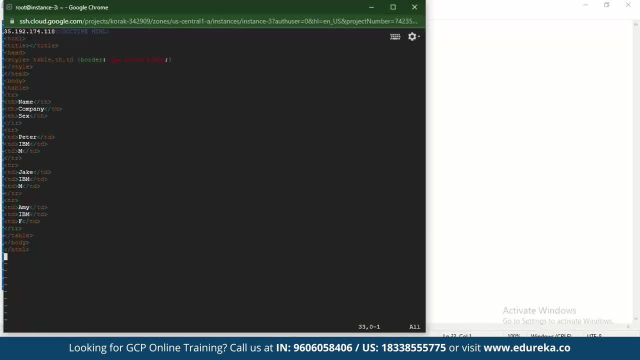 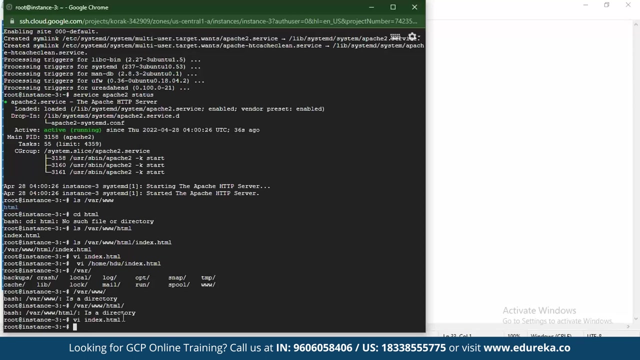 right. so you just have to vi into the indexhtml right, take your code here, copy it and end in here. so right now you have your code and it's changed from the apache page to your very own web page, right the command, column WQ. so now, when you refresh this, let's just try refreshing. 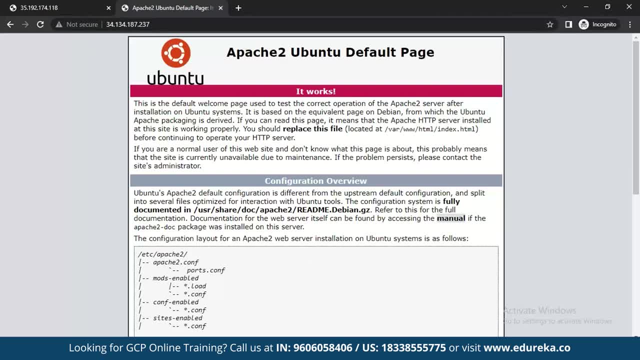 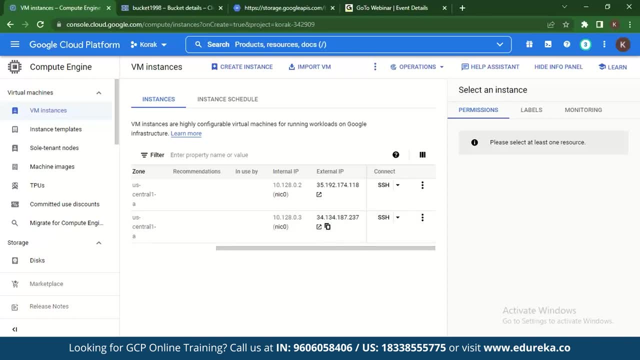 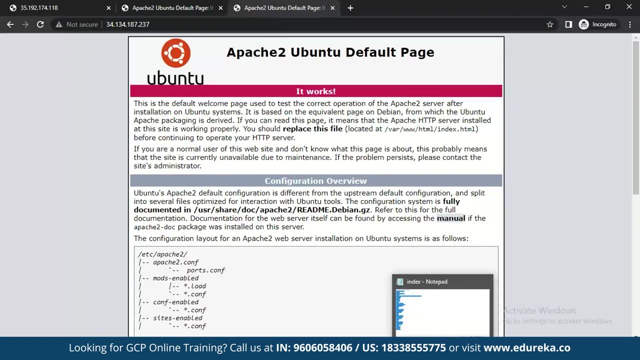 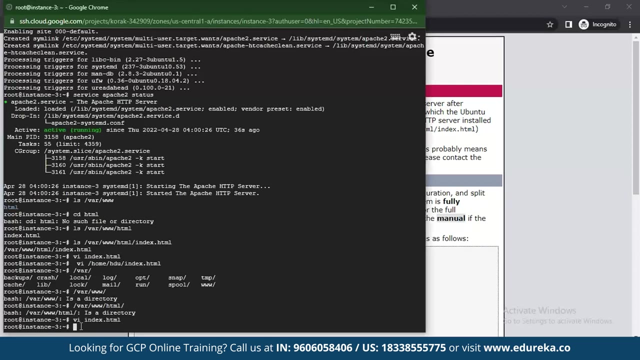 this, it's still the same, and let's go back to our right. so copy this up. is this? add it, and so what you have to do here is starting from change the HTML code. so, now that you've changed the estimate code, what you need to do is 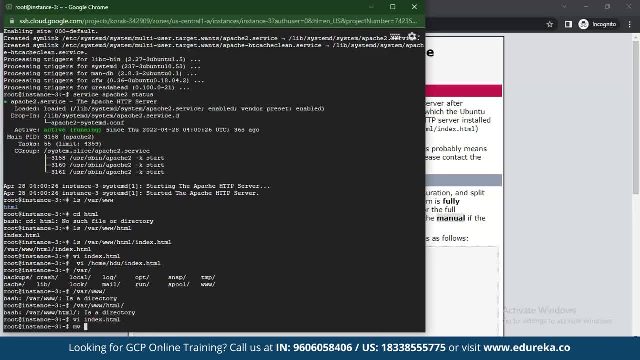 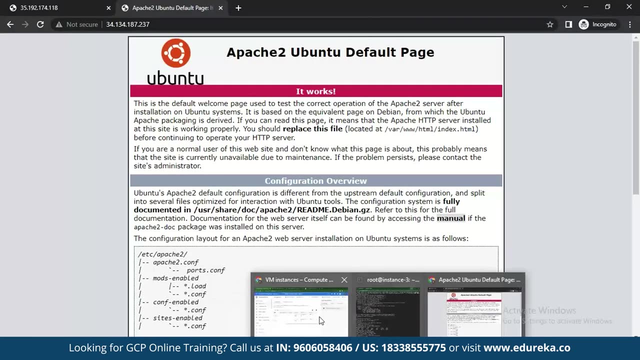 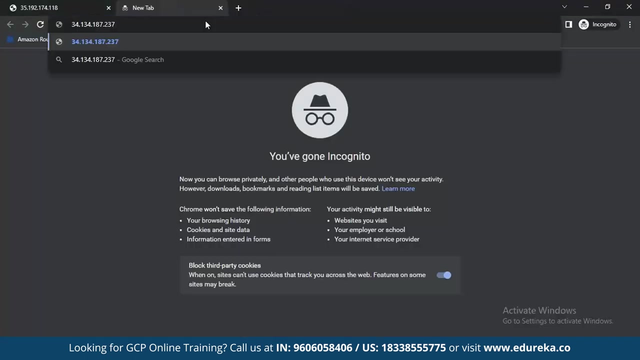 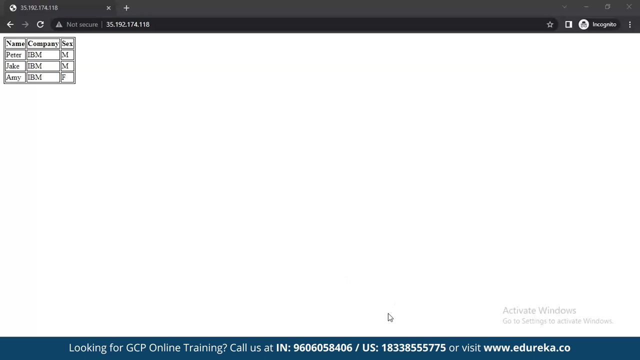 move it in somewhere else. let's try this. and we index dot HTML, index one HTML. so now let's try it out. go back here. this and this is this, and basically what you see is that you have your own web page in here, which you replace with the Apache web page, and that is because you went into the SSH. 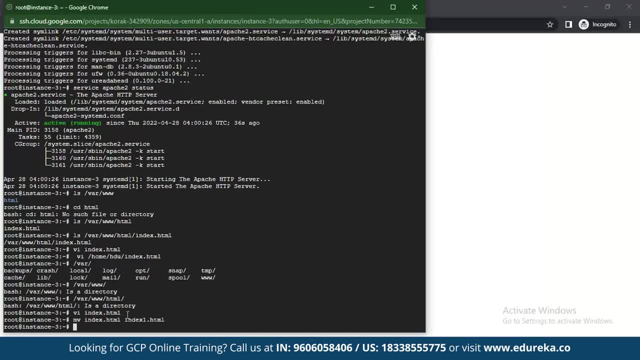 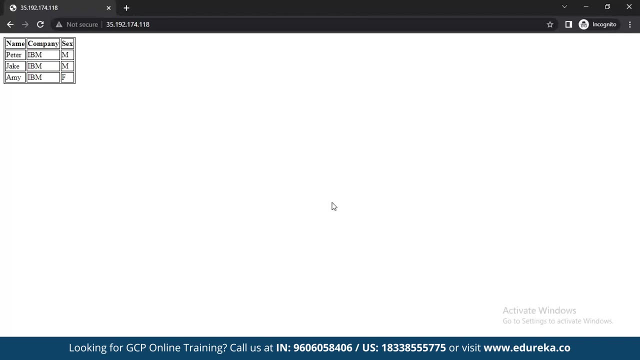 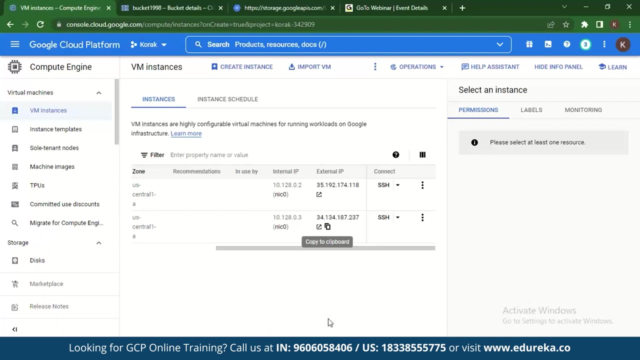 change the code in index dot HTML and move it from index to index one dot HTML. so that is basically how you host a dynamic website using servers and in VMS on Google Cloud Platform. there's another way you can host dynamic websites on Google Cloud Platform, but that is through App Engine. 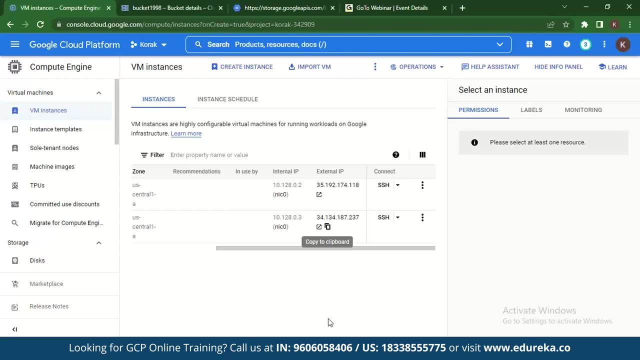 if you would like us to make a video on Google Cloud App Engine, please do let us know in the comments below. and now let's go back and check out what it's like to host a static website, right? so when you create a static website, you need buckets. 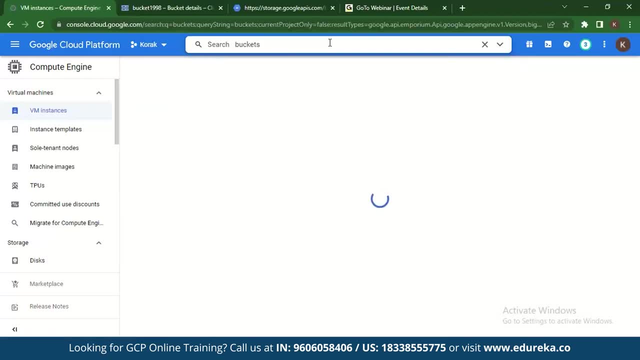 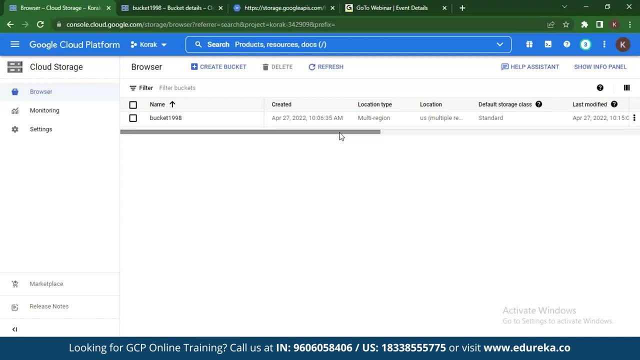 and what you need to do is just go to cloud storage. so when you're talking about hosting a static webpage, you basically need only a storage service, because you're going to basically get HTML code in these storage buckets and these buckets have then got a URL which are publicly accessible, and you'll have 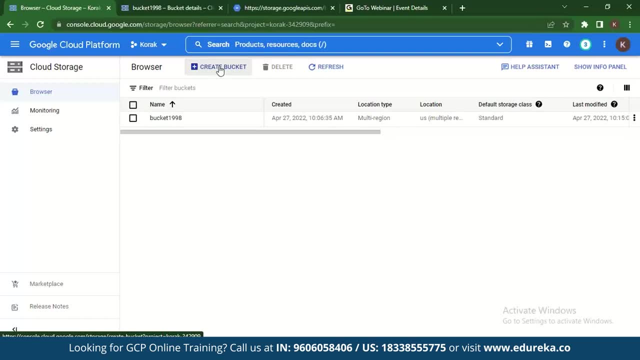 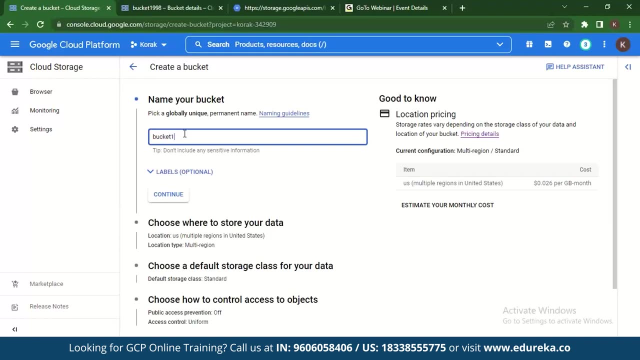 hosted a static web page, so let's get started with a static web page. We'll try and create a bucket, So I name it anything we want, Let's say bucket 997,. right, Continue. Okay, so this is taken. So let's try this out, right. 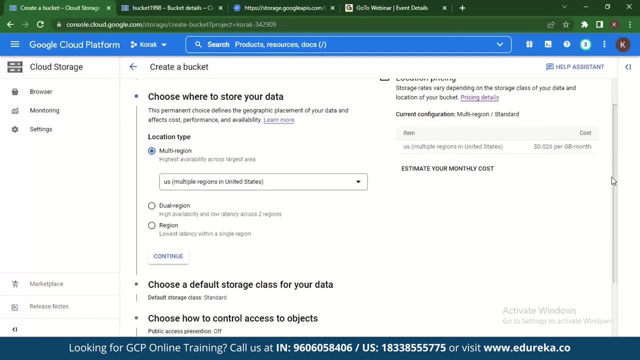 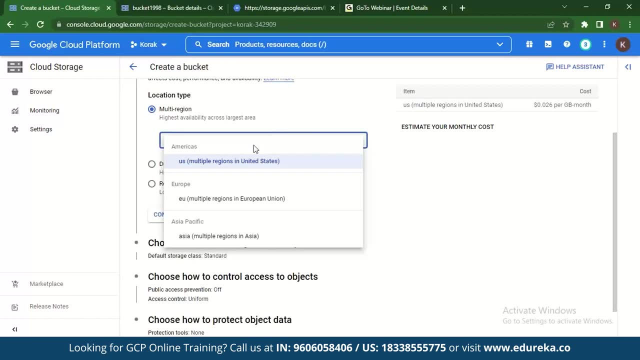 So we want it to be multi-regional because it will be publicly accessible, right? So this is going to be multi-regional and US- multiple regions in the United States. right, So you can change it to Europe if you want. Let's go to continue again. 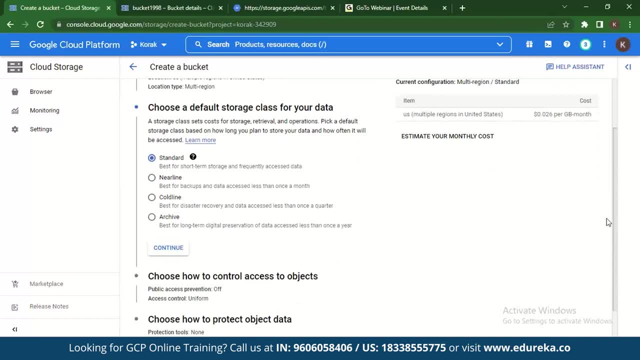 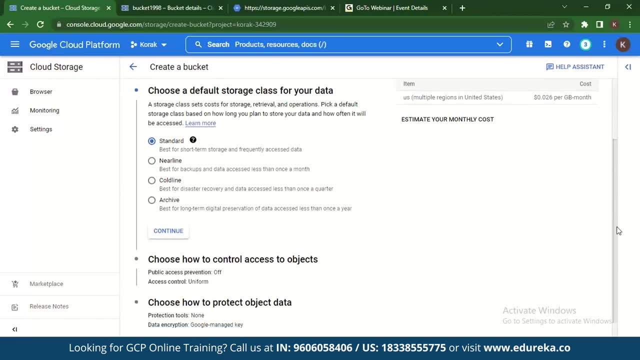 You get to choose your default storage class for your data, And these are divided into standard, nearline, coldline and archive, Standard being the most short term and archive being the most long term. And then let's go to continue. So what do you want to do? here is? 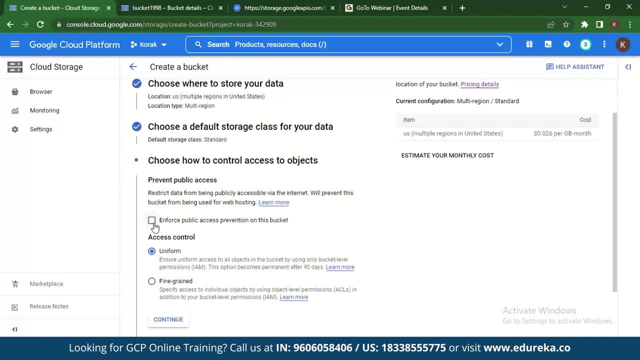 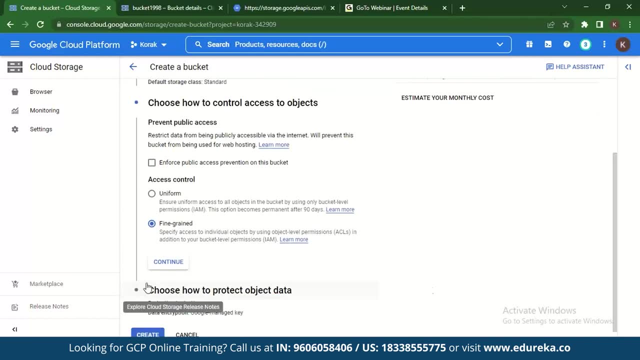 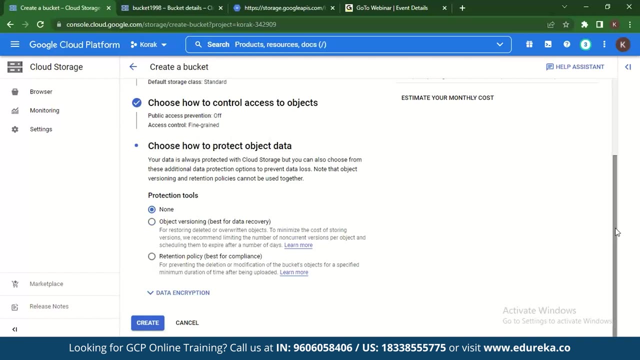 we don't want to prevent public access, right, So we'll not take on this. What we'll do is give it to fine-grained, where we'll have ACL permissions, and go to continue, And what we'll do here is have none of the protection tools. 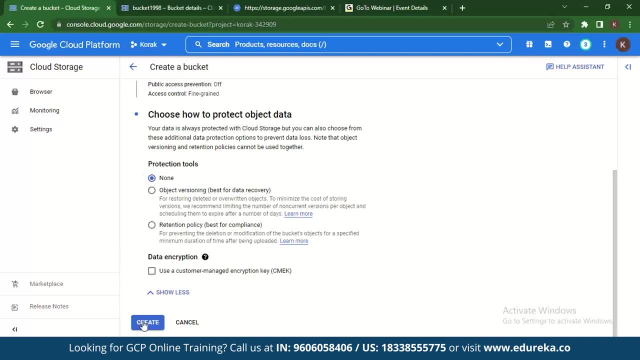 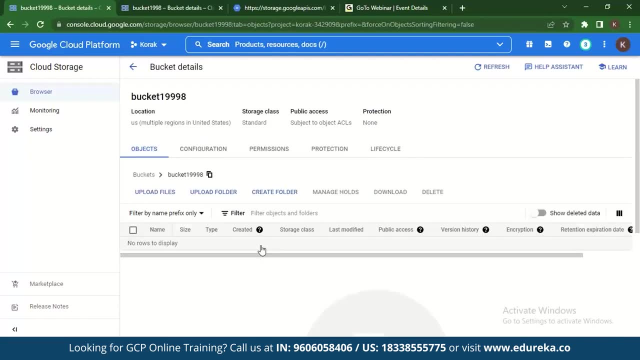 but we'll have none of the protection tools, And right after that we'll basically create our bucket. Right. so our bucket is created. Now what we need to do is upload our HTML pages in the bucket. on this bucket, Let's do this. 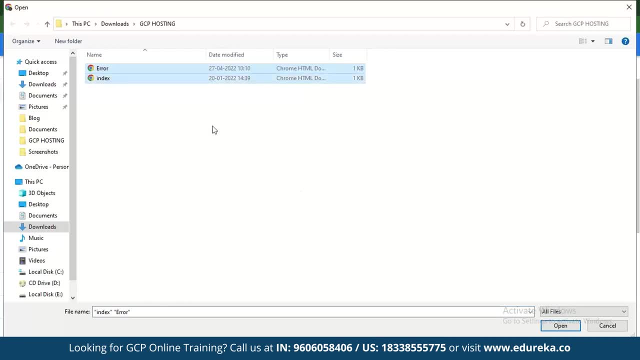 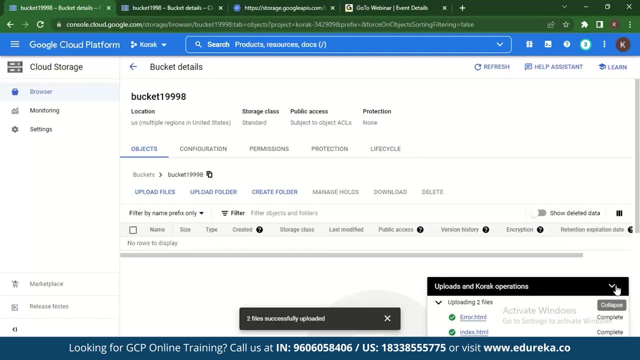 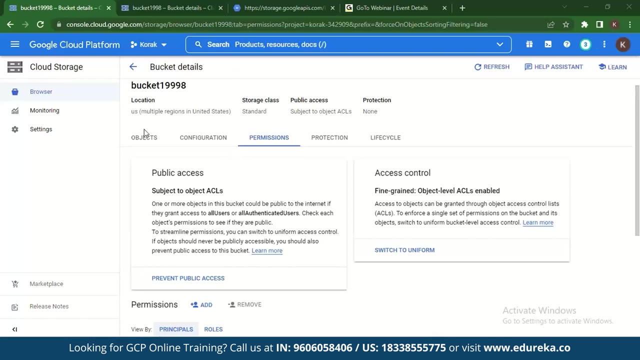 There's an error file I have and there's an indexhtml file I have. Let's upload both of these. So we've uploaded both of these files. So, basically, what we have to do now, after we've created the bucket, is change its permissions. 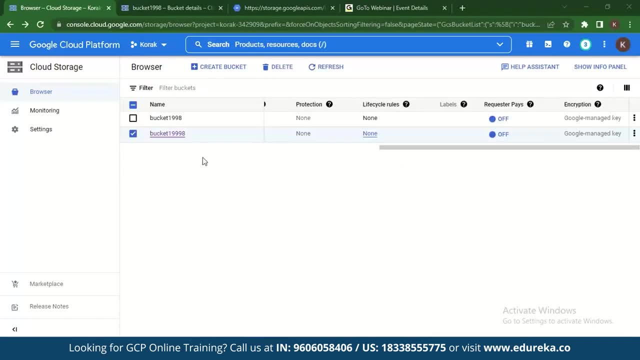 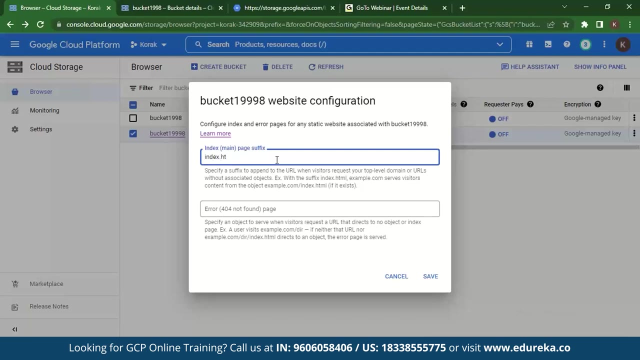 and allow public access. So once you've basically made the bucket, you have to change the configurations- that is basically edit website Configuration- and you have to add your indexhtml and errorhtml and save it right. So right after you've done that, 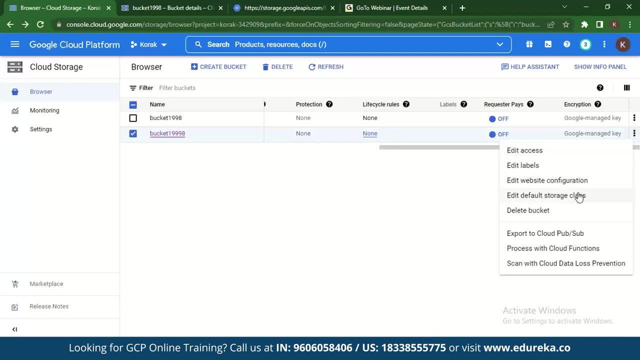 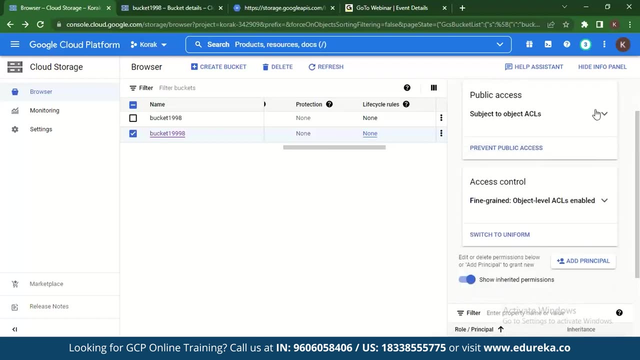 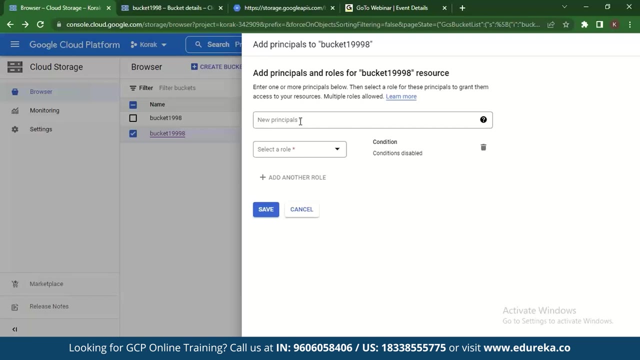 last thing you need to do is you have to edit the access. Now, when you're editing the access, you need to public access Next to ACLs. now, what we'll have to do is add a new principle, and here we'll have to. 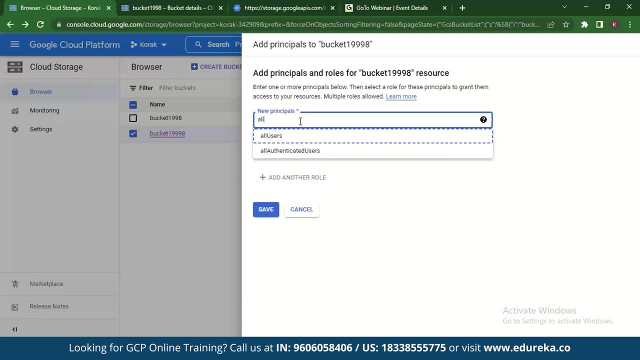 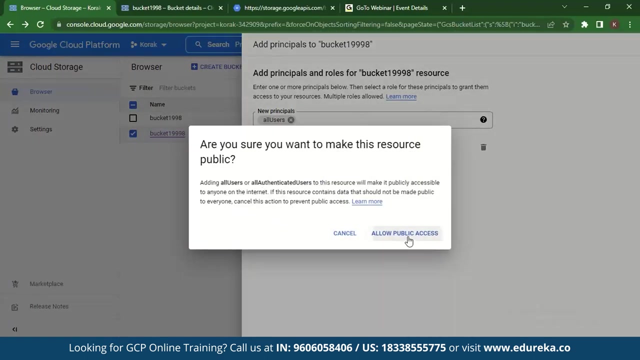 select all users right and here to here we'll have to select a role, which is the object view storage object viewer, which basically gives you the view access to the website only, and you have to save that. so, basically, this is asking if you want to make it public. so we just have to update this and now our bucket has. 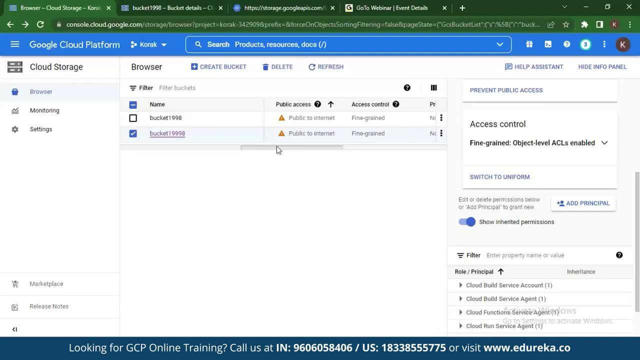 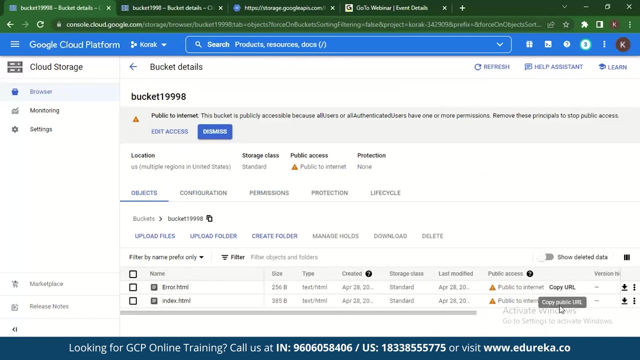 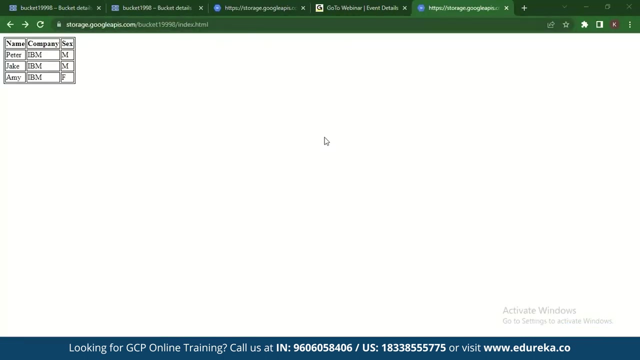 public access. let's just check. right? so there is public access to the internet, right? so now that we have public access to the internet, let's just go check out our URL. so enter your bucket, copy the URL and paste it in here so as you can see our indexhtml page. 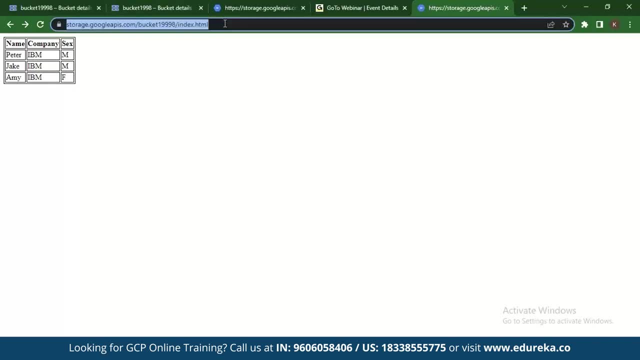 has been posted on this endpoint, which is basically googleapiscom, with this bucket name: indexhtml, and that is how you host a static website on Google Cloud Platform. so we've seen how to host a static website and we've seen how to host a dynamic website. so 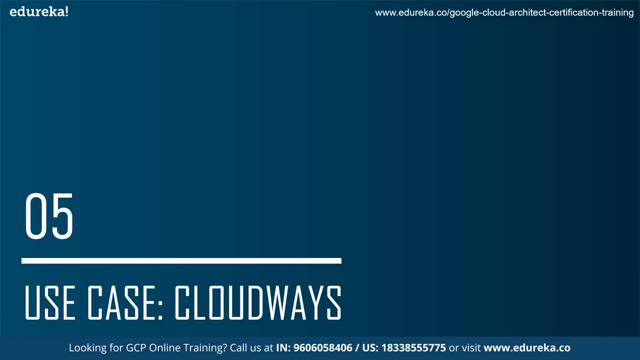 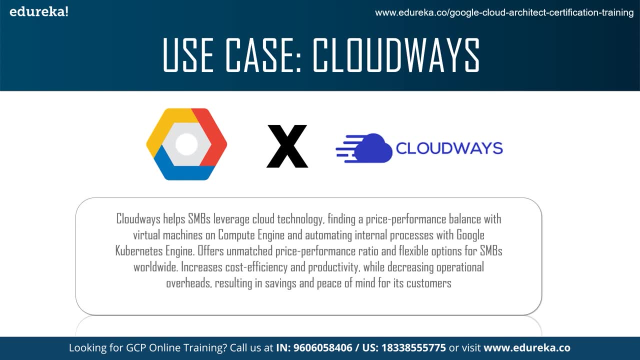 the last thing we talked about is the use case. so, when it comes to the use case we talk about, we're going to talk about one very popular use case, which is the cloud ways use case. so cloud ways is basically in partnership with Google Cloud Platform and what happened is the price performance balance for the 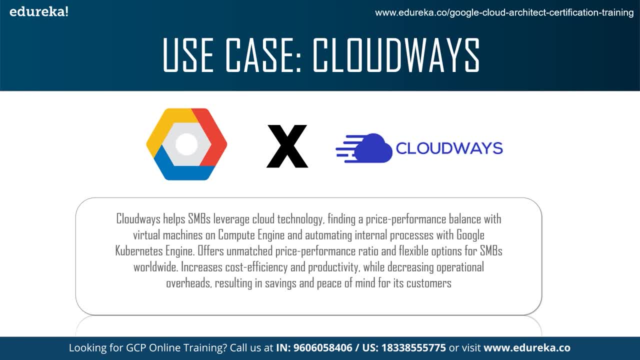 virtual machines, cloud computing engines, automatic compute engines, repeat automating compute engines, internal processes, Raven of crowd ways in collaboration with GCP has improved. in fact, a lot of 動 falls class 됩니다 already existing services, such as the cubilities engine, the computer engine and other search performance ratios, and this basically. 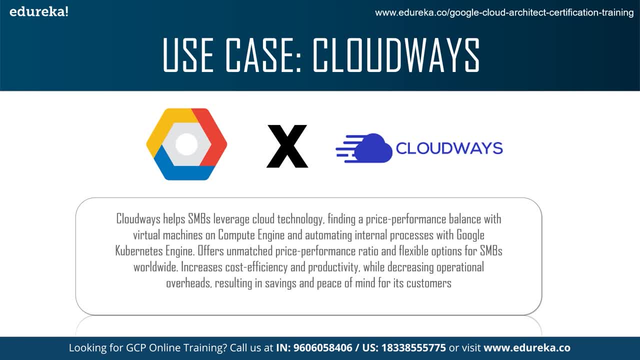 increases a lot of cost, efficiency and productivity. right, so this is how bursting using our cloud Googleadt platform has a lot of the connectivity in there, which enhances efficiency and productivity. right, so this is how hosting using cloud platform has an enhanced and this basically increases a lot of cost, efficiency and productivity. right, so this is how posting using cloud Google platform has an enhanced. 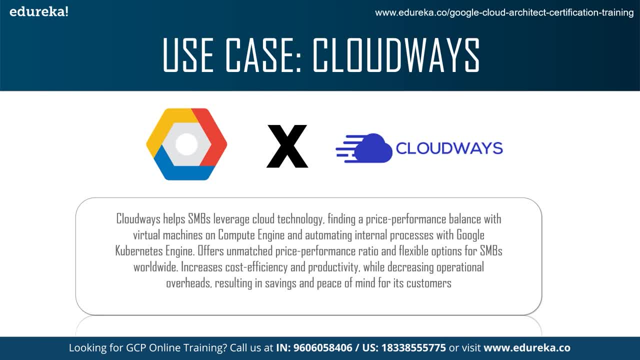 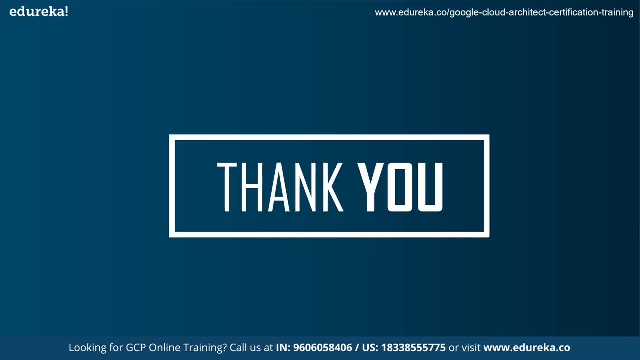 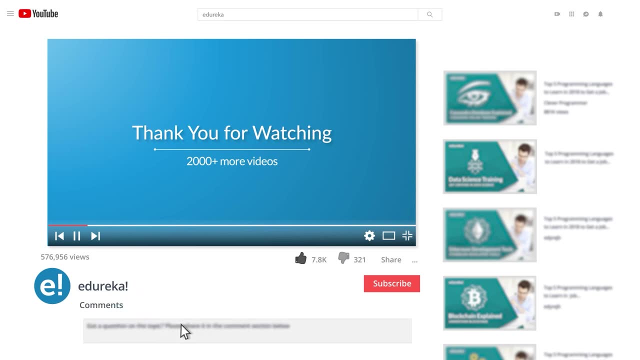 made cloud raise much more scalable and cost effective, right, so with this we come to the end of the session. thank you and have a nice day. i hope you have enjoyed listening to this video. please be kind enough to like it and you can comment any of your doubts and queries. 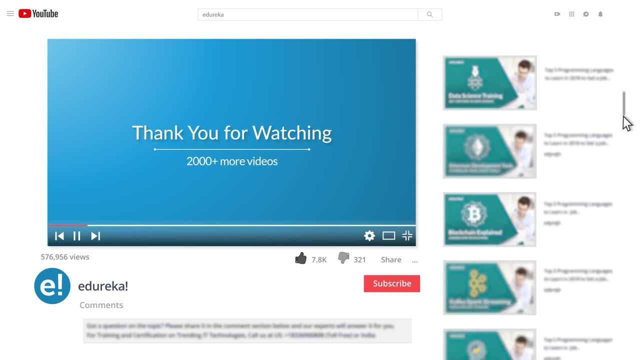 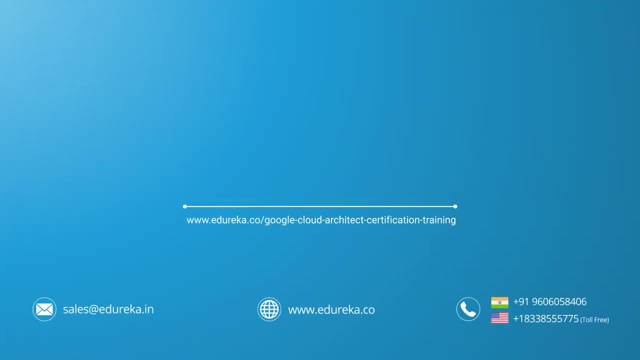 and we will reply them at the earliest. do look out for more videos in our playlist and subscribe to edureka channel to learn more. happy learning you.